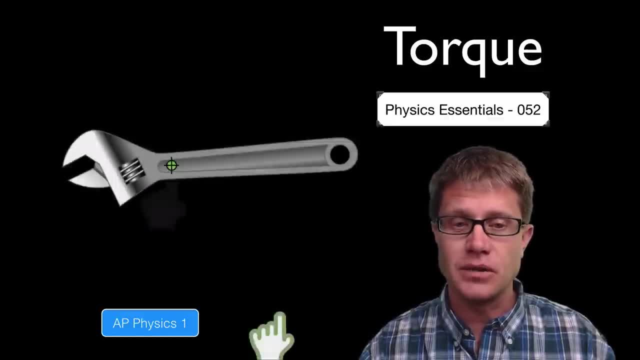 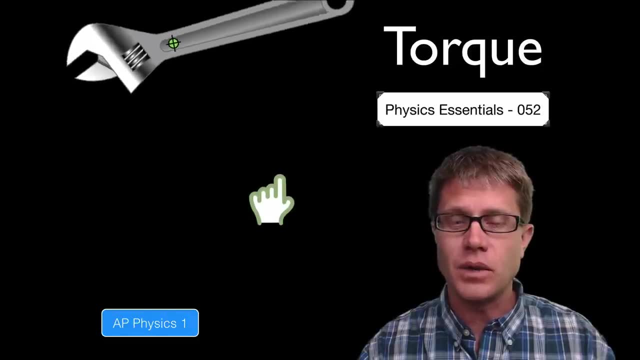 We apply a force in one direction and we are seeing an acceleration in that direction. Let's say I do the same thing, but now I am going to do it off center, So I am applying a force not at the center of gravity And watch what we get. We get two forms of motion. 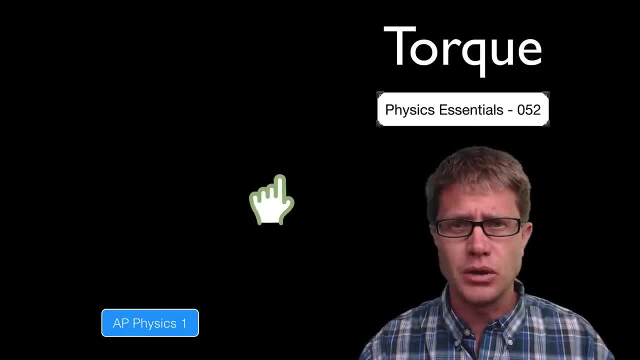 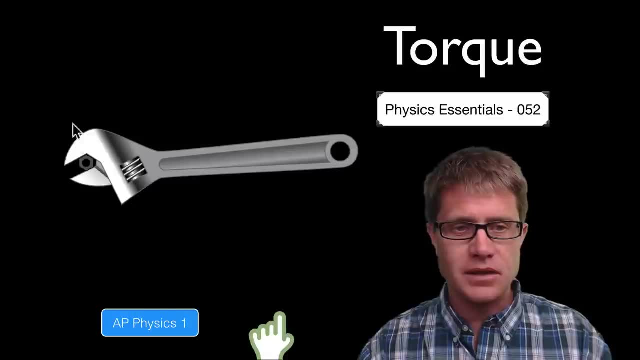 We are getting that translational motion, but we are also getting rotational motion, And it is hard to separate those two, And so an easy way to look at rotational motion is to pin it down. So now I have got this same thing. We have got the wrench, but now it is centered around this nut on one side. 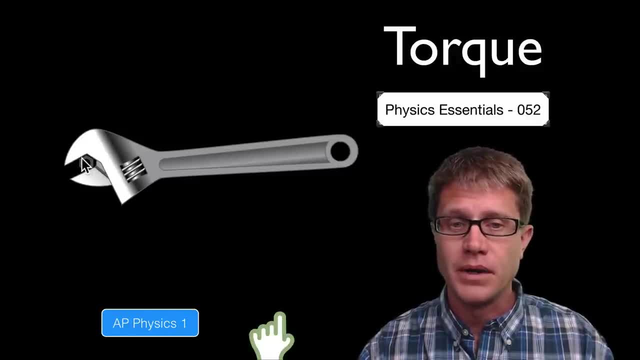 And so this is not moving, So it is going to rotate around that point. Now let me apply that same force on one direction, And now we are just getting that rotational motion. Let me return the wrench for a second and we can start to talk about what torque is. 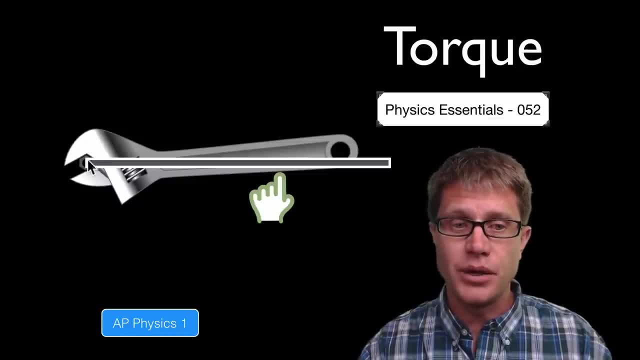 And so this is going to be the lever arm. The lever arm is going to go from this point in the middle that axis of rotation. It is going to go out from that That is perpendicular to that axis of rotation, And it is just like a lever that you would. 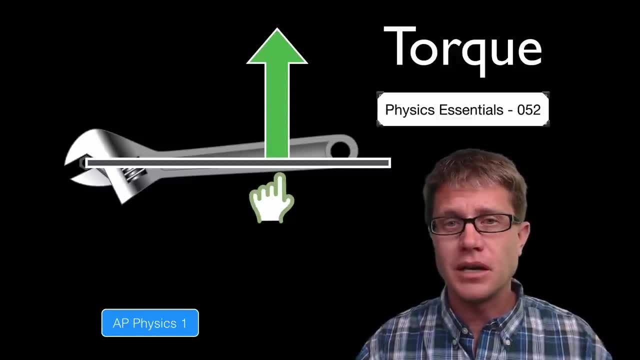 use as a simple machine. And then we are applying a force perpendicular to that lever arm. And so what is torque? We are multiplying these two values, We are multiplying the force that we apply perpendicular to the lever times, the lever arm itself, And so it is two things. 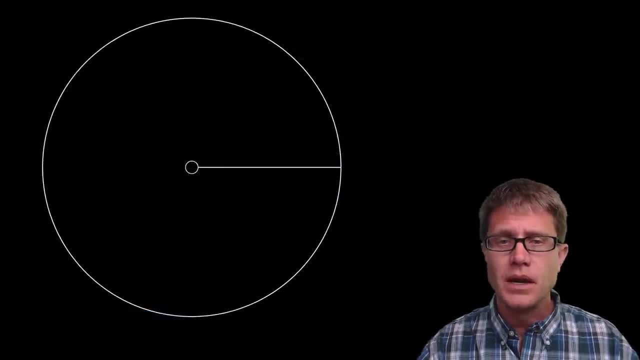 And the units are not just going to be newtons, It is going to be newton meters. And so in a rotational system like this, where we have an axis of rotation, what is torque? It is simply the product of that lever arm which is going to be a vector and has to be perpendicular. 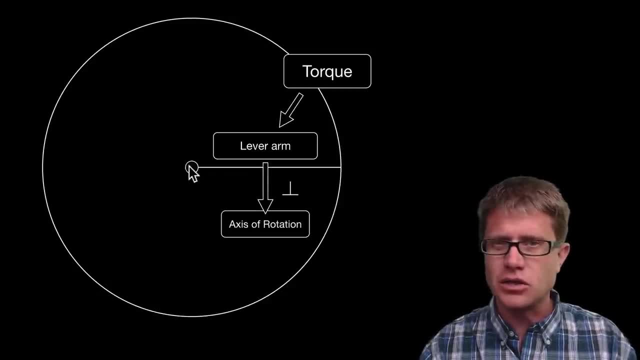 to that axis of rotation. Again, the axis of rotation is coming straight at us through the middle And we are going to multiply that times the force. The force has to be perpendicular to that lever arm, And so if we multiply those two values, then we are going to have ourselves. 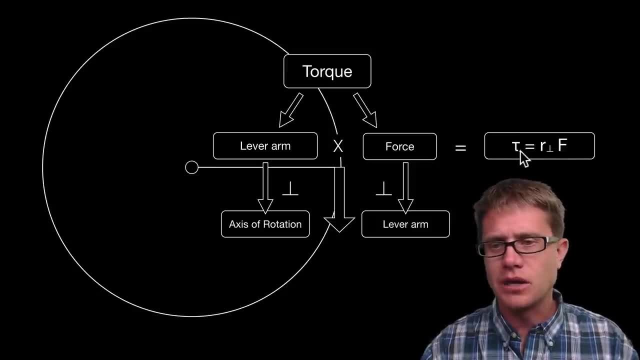 a torque, And this is our equation right here. Tau, which stands for torque, is equal to that lever arm, perpendicular, and then that force. And so if we have a system that is not moving, like our rotational system is not moving anymore, 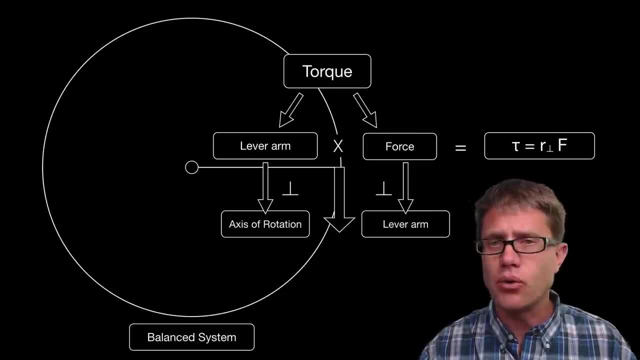 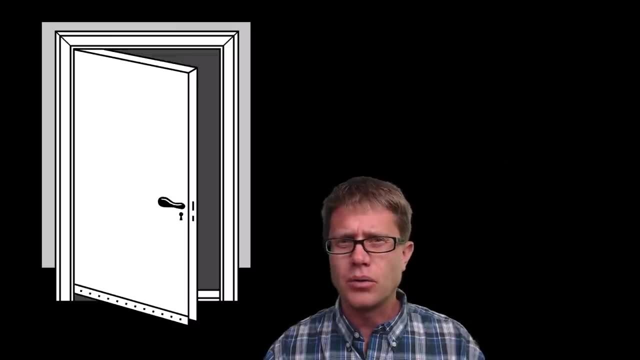 we know that all those forces must be balanced, In other words, all the torques must be balanced, And so the net torque on a balanced system is equal to 0.. Have you ever noticed that a door will always have the doorknob on the outside or far away from the hinge? Well, the 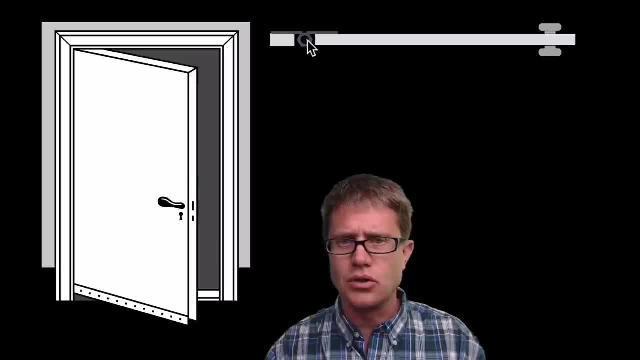 reason that is just deals with torque, And so what I have here is the door itself. This is the door hinge right here And here is the doorknob on the outside. And so if I have a lever arm, what happens if I apply a force out here? What am I going to get Torque. 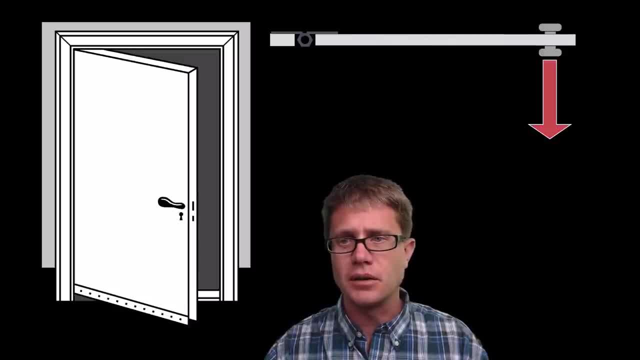 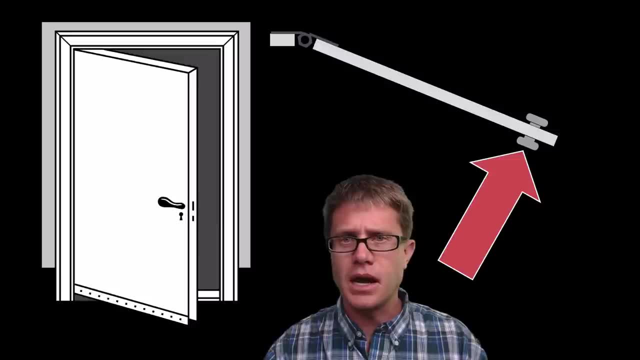 We have got the lever arm and then we are applying a force perpendicular, And so we are going to get an acceleration or a rotational acceleration, like that. What happens if I apply a greater force? What am I going to have? I am going to have a greater torque. 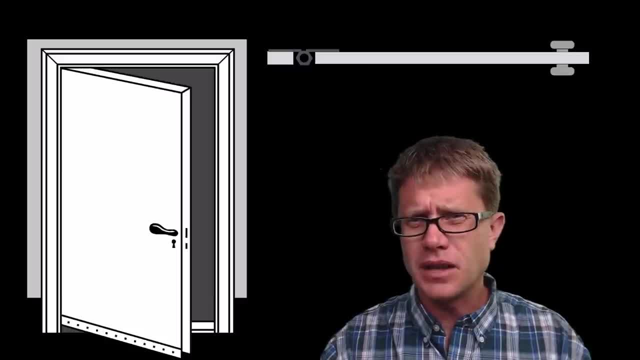 And so we are going to see a faster acceleration like that. What happens if I take that smaller force, however, and move it to the inside? What happens if I put the doorknob on the inside of the door, If I try to pull on it with that small force? nothing will happen. 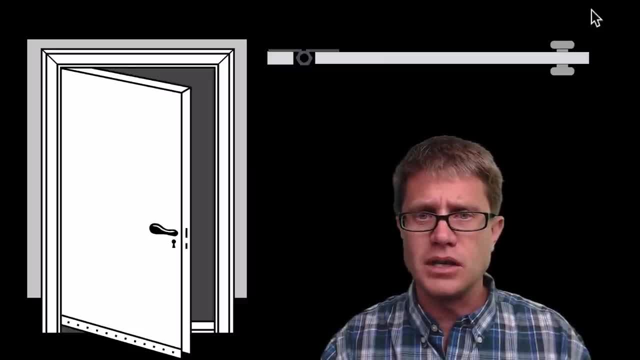 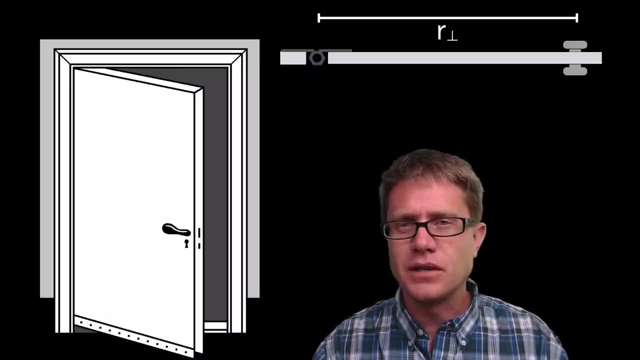 In other words, I have decreased that torque so much, since I have decreased that lever arm, that I would not have enough torque to open that door, And so that lever arm distance is incredibly important. Just like a lever in a lever system, it is giving us a mechanical 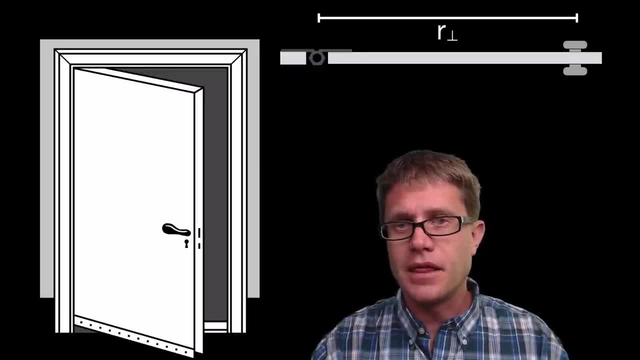 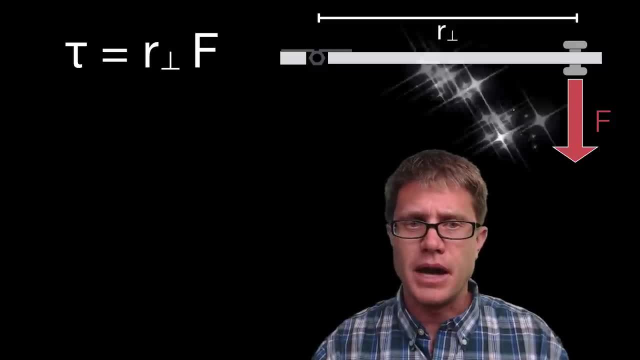 advantage to open up that door. So in torque we are applying that lever arm times the force. That is how we calculate the torque, And the equation looks like this: Tau is equal to R perpendicular F, And so let's add some numbers in here and I will show you how to calculate. 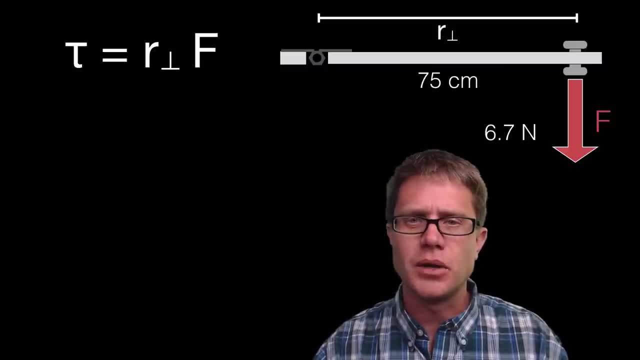 that Let's say the doorknob is 75 centimeters from the hinge and we apply a 6.7 newton force. What is going to be our torque in this situation? Well, I am going to plug in those values Again. 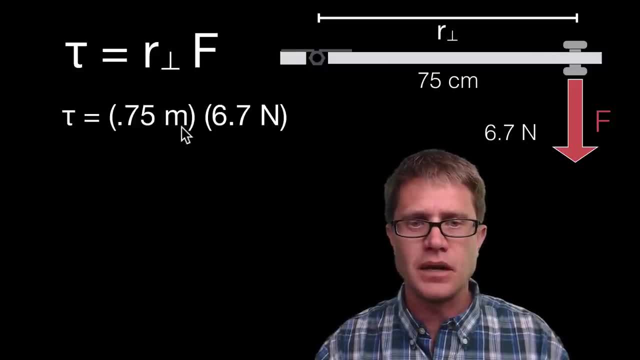 I had to convert these centimeters into meters. We have to use SI units And now I simply multiply those values. What are my units? It is now in newton meters. You can see I have too many significant digits, And so we would get a 5.0 newton meter torque if the 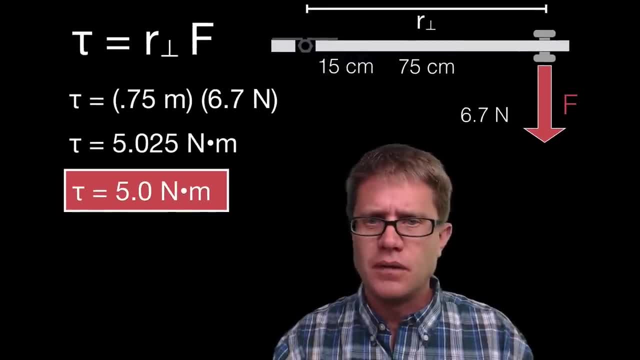 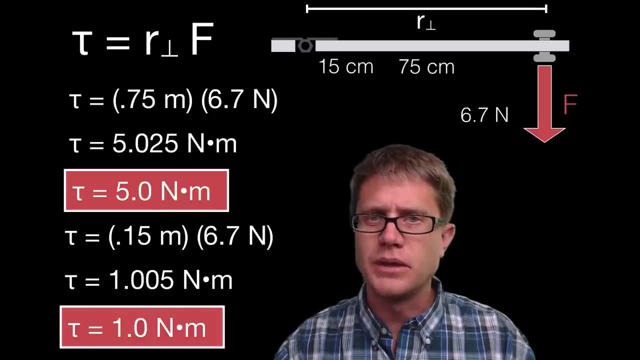 doorknob is at the outside. Now watch what happens if we move it 15 centimeters from the hinge. Watch what happens to our torque. Again, the force is going to be the same, But now we are going to get a 1.0 newton meter torque. It is one fifth what it was before. 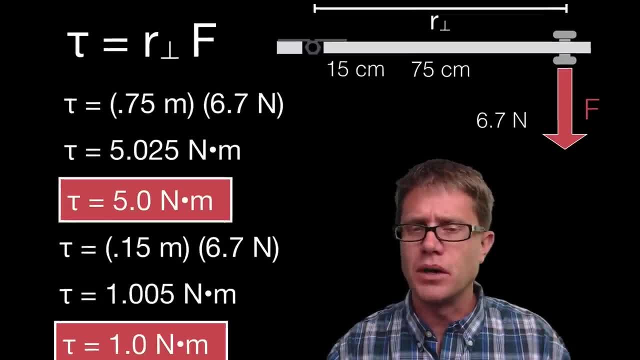 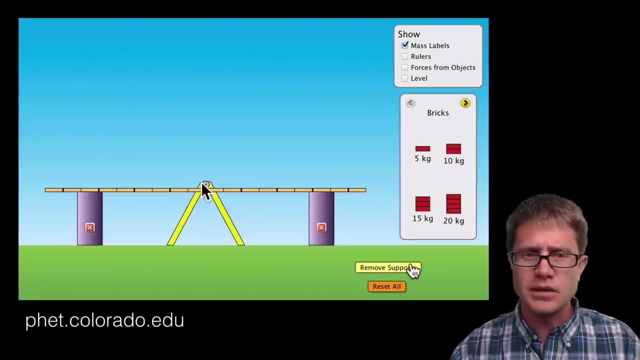 Which isn't surprising, because the lever arm is now one fifth what it was before. Let's take a second to look at a balance system, And a seesaw or a teeter totter is a great example of that. We have the axis of rotation right here in the middle And we can have 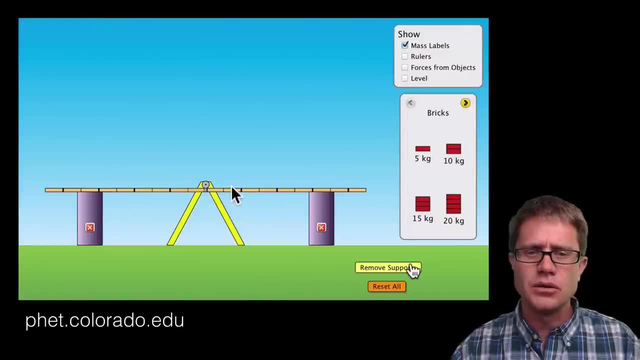 a lever arm on this side and a lever arm on the other side. So what we can do is we can apply a torque on one side and a torque on the other side And what we are going to do side, And if those torques are equal, then we are going to have a balanced system. We 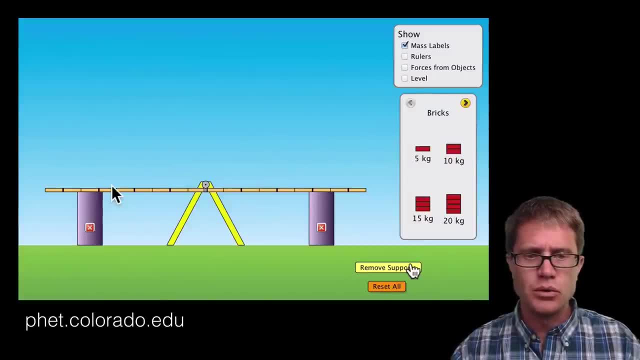 should not see any movement, And so watch what happens when I remove the supports. Since the torque is the same on either side, nothing happens. Let me apply a 5 kilogram weight on either side. If I remove the supports, it is totally balanced. Torque is equal on. 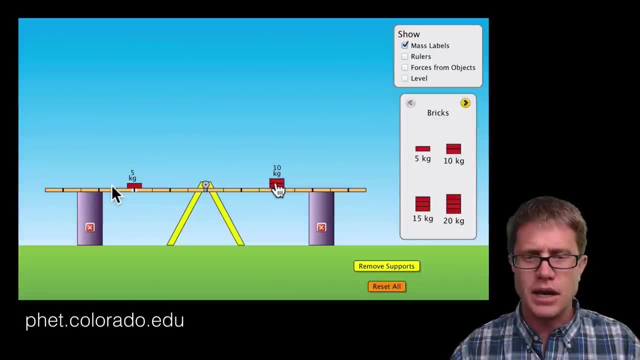 either side. Let's say I add a 10 kilogram weight to the right side and now remove the supports. What happens? Well, we have got greater torque on the right side, And so we are getting rotational motion in that direction. Now, a good question I might ask you is: where could 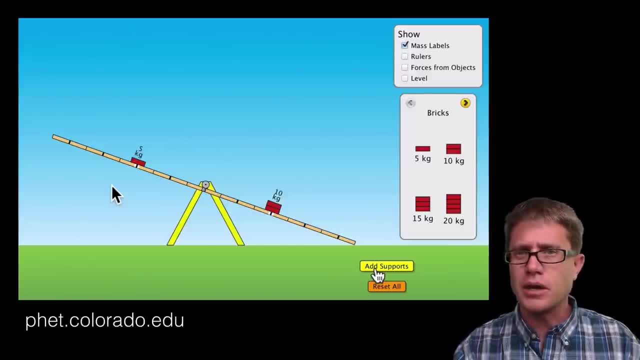 I move that 5 kilogram mass on the left side, so the torque on the left equals the torque on the right. How could I balance this system out? Well, if we look at our equations again, it is simply the product of the lever arm times the force, And so if I throw in some 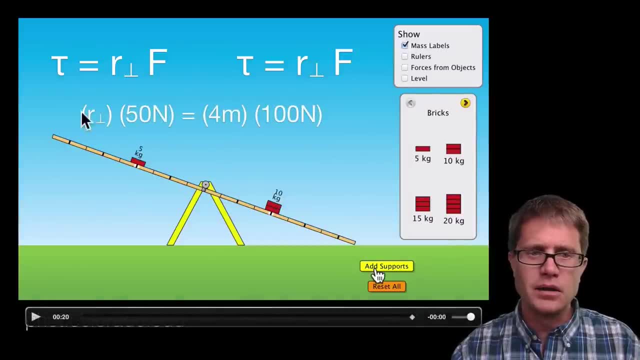 values here and set them equal to each other. on the left side we have the unknown lever distance times, that 50 newton force, And so if I move that 5 kilogram mass on the left side, where do I get the 50 newton force? I am simply taking 5 kilograms times about. 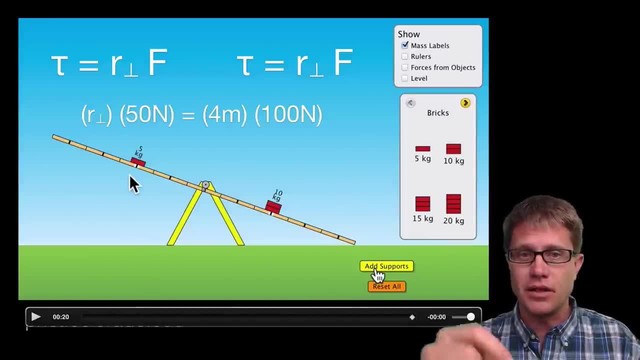 10 for the acceleration due to gravity. So it is a 50 newton force down on that side. On the other side it is going to be 100 newton force. So I could solve for this. We would have a torque of 400 newton meters on the right side And so to solve for that we should. 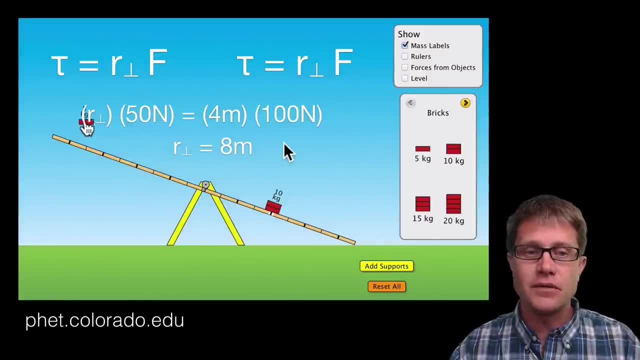 have a distance on the left side equal to 8 meters, And so if I take that 5 kilogram mass, move it out to 8 meters, what are we going to get? A balanced system. The torque on either side is going to be exactly the same, And so did you learn the relationship. 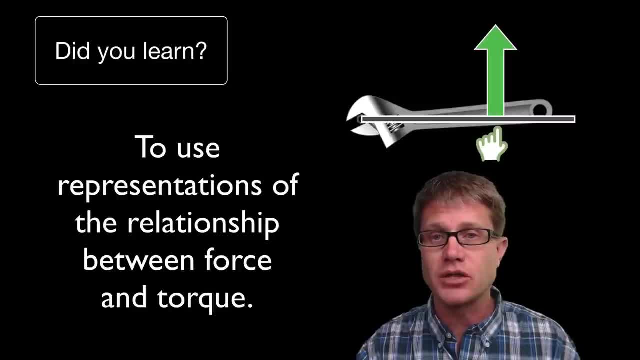 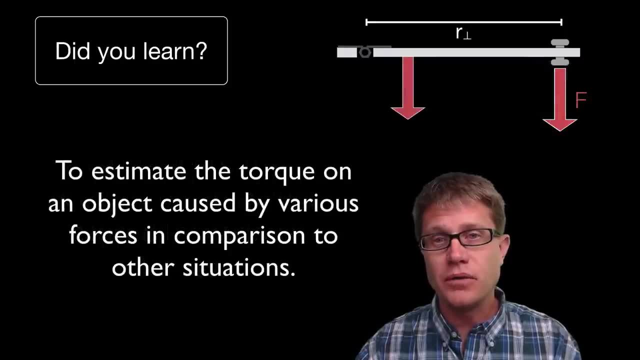 between a force and a torque. Again, we have to multiply the force times that lever arm. Do you see what happens when we apply different forces? We increase the torque. Or what happens if we move that force in? We are decreasing the torque because we are decreasing the lever.